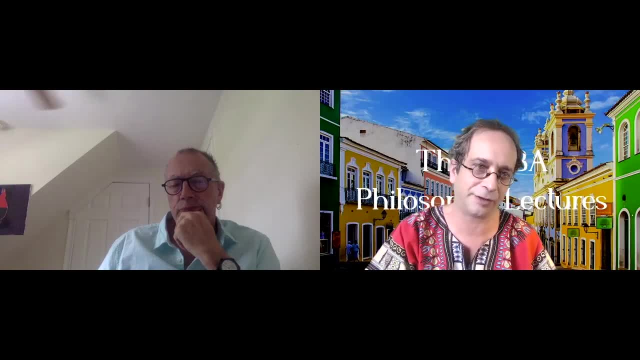 was to conceive of them as the extension of concepts, And we discussed how Russell pointed out that this didn't go any way because it contained a contradiction. So if logic was to survive, something had to be done, And between 1910 and 1913,. 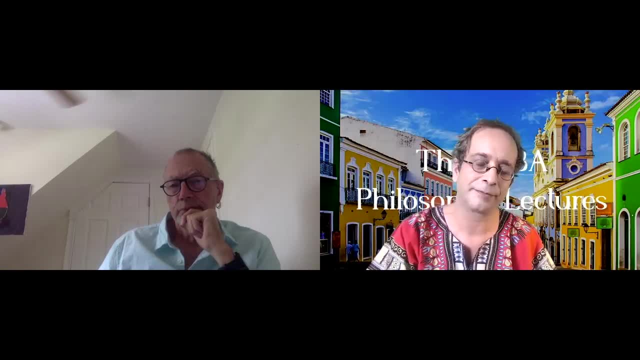 Russell, together with his colleague Whitehead, wrote the Principia, which are, in a sense, a bible of logicism, And I would like you to tell us what they succeeded in doing and what kind of conception of logicism emerged out of their work. 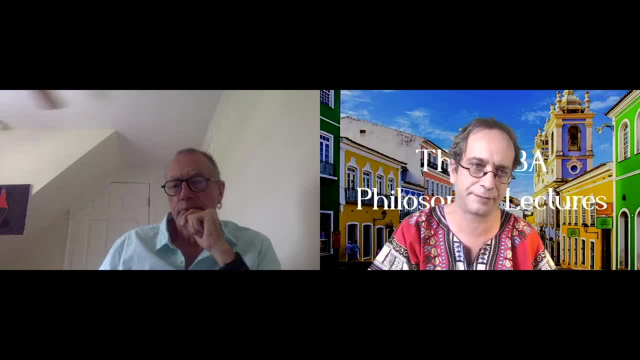 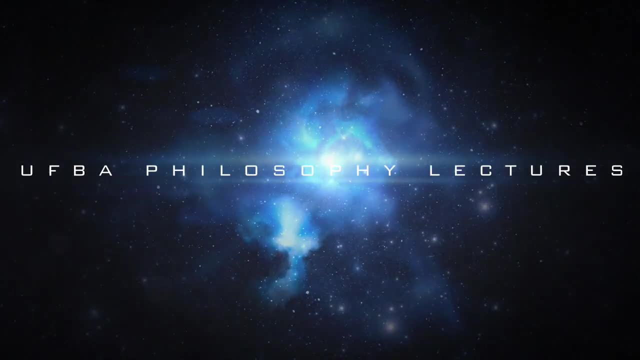 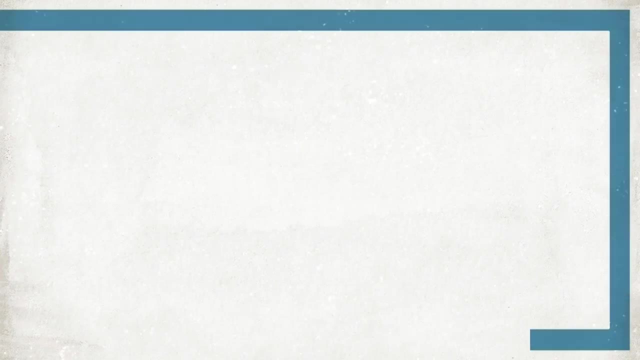 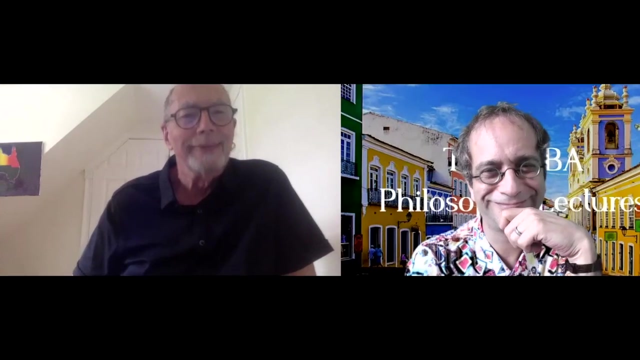 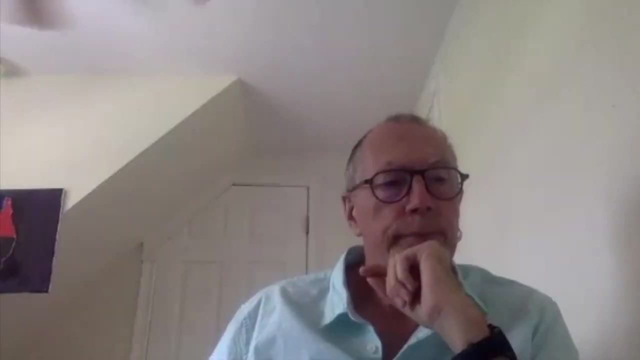 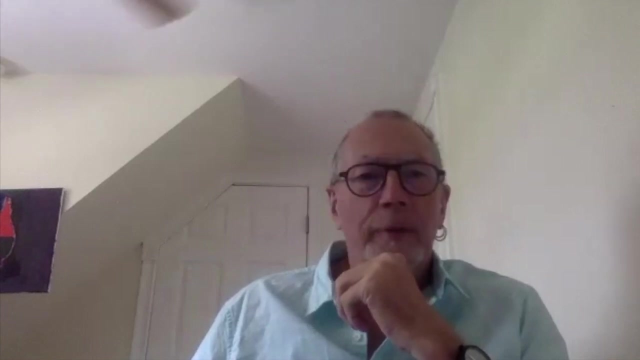 and how it differs from Frege's conception. Okay, well, you're right that Frege and Russell were logicists in the sense that they thought you could reduce some mathematics to logic. Whitehead, I think, was just only ever a technical guy. 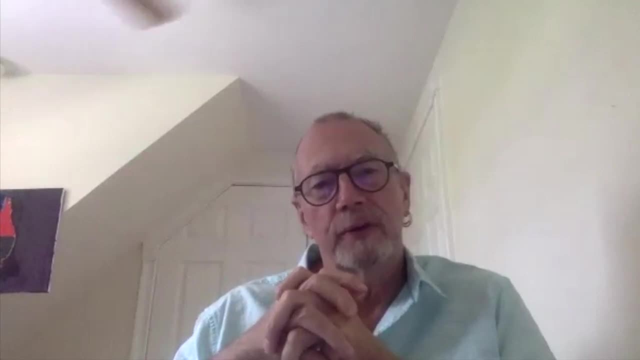 at this stage of his proceedings, so I'm not sure that he had a philosophical view. then There is a difference between Frege and Russell, because Frege thought that you could reduce arithmetic and analysis and so on to logic. He thought, if I remember right: 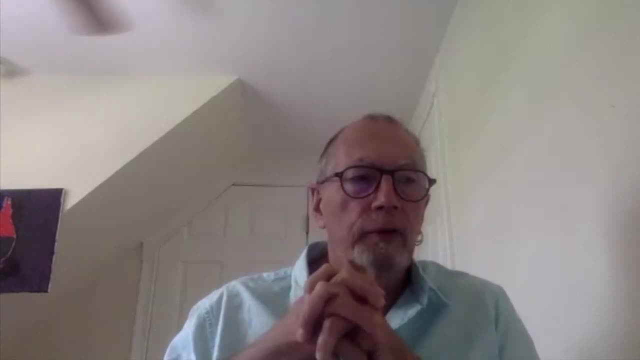 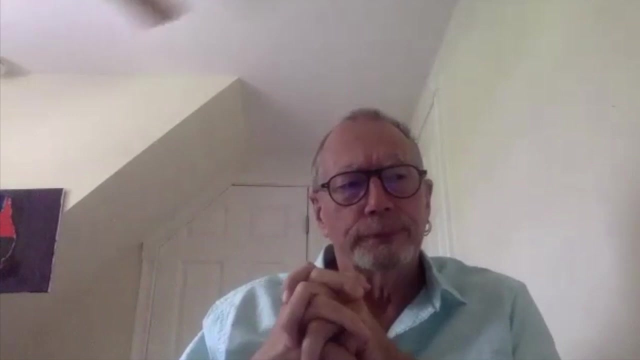 that geometry is synthetic, Whereas Russell's claim was more ambitious. Russell thought that you could reduce all mathematics to logic, including geometry. And if I again, if I remember right, well, there are only three volumes of Principia which were published. 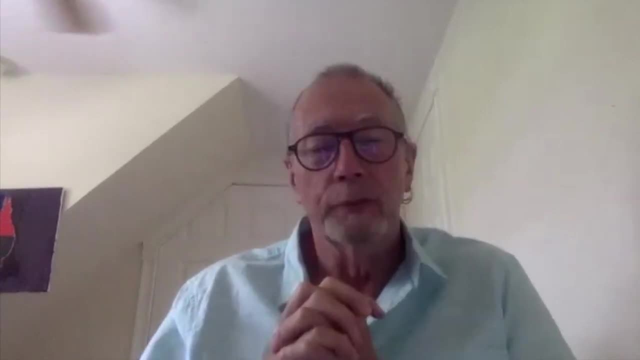 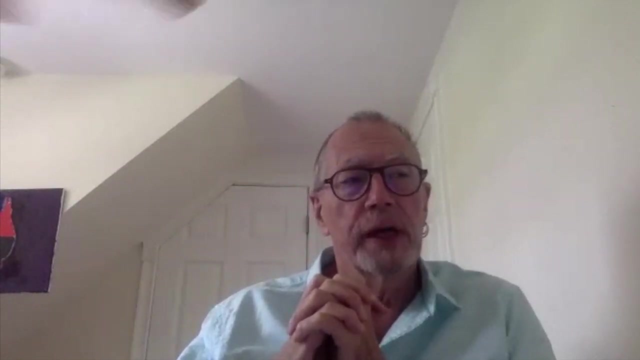 There was a fourth that was slated, and I think that was due to be written by Whitehead, in which geometry was reduced to set theory. That was certainly never written, So that part of the project remained incomplete, as it were. However, that's sort of a side issue. 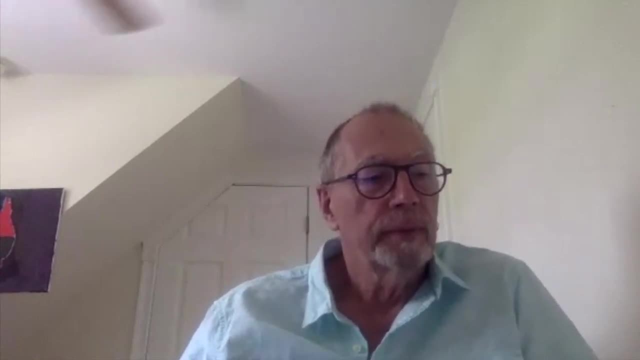 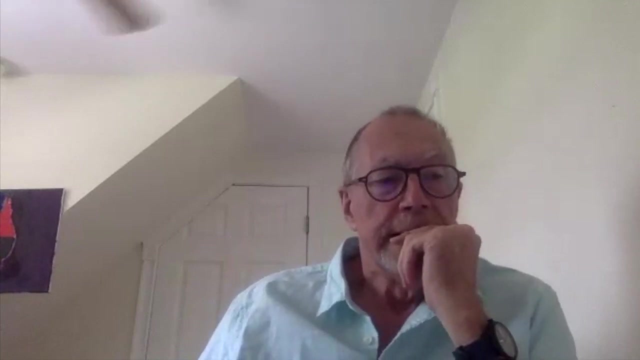 because the question is whether, even in the first three volumes, Russell and Whitehead succeeded in reducing arithmetic analysis and so on to logic, And they had the problem of the inconsistency of set theory to deal with. So it's true that Frege thought he was reducing arithmetic to logic. 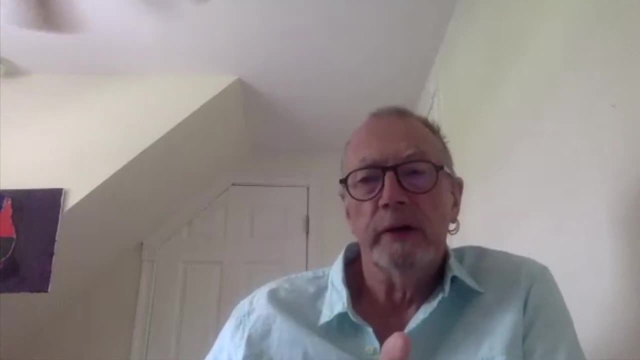 but he did have axioms which were effectively about sets, But they looked kind of general enough to be the sort of thing that logicians could deal with. Because of Russell's paradox, you could no longer accept these axioms, Or at least. 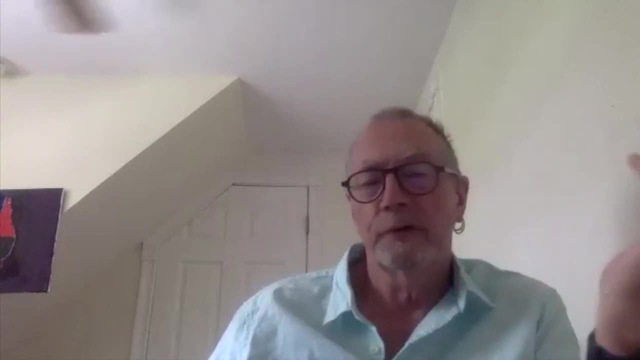 you could no longer accept these axioms. if you apply classical logic, that is sort of Frege and Russell logic. So you have to change your set theoretic axioms And it's not at all obvious how to do this. So this is a problem. 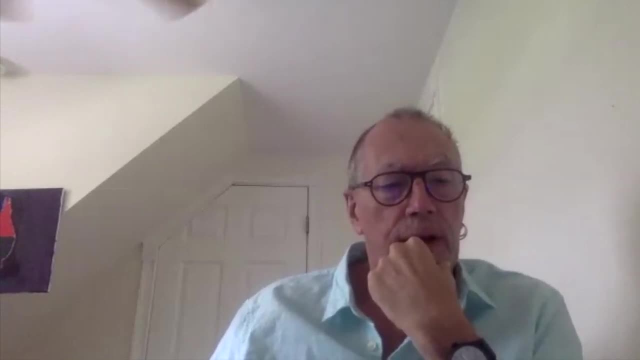 that Russell struggled with for a number of years. I mean, he discovered his paradox in the early years of the 20th century And I don't think he found a solution that satisfied him until about 1908.. And in his autobiography. 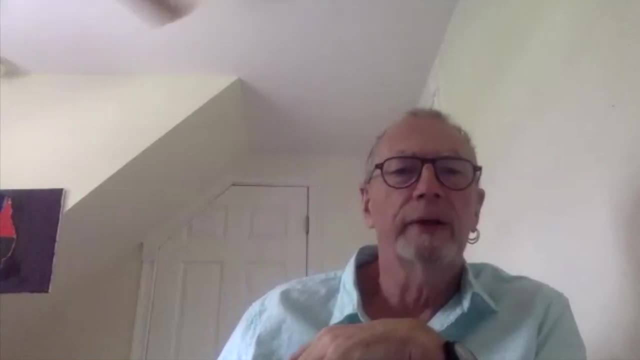 he tells us that he was living in Bloomsbury in London at the time, I think, And there were many days when he would get up, have breakfast, go and sit in his study with a blank piece of paper in front of him. 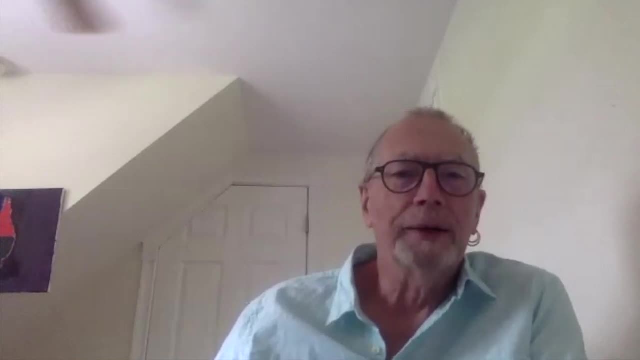 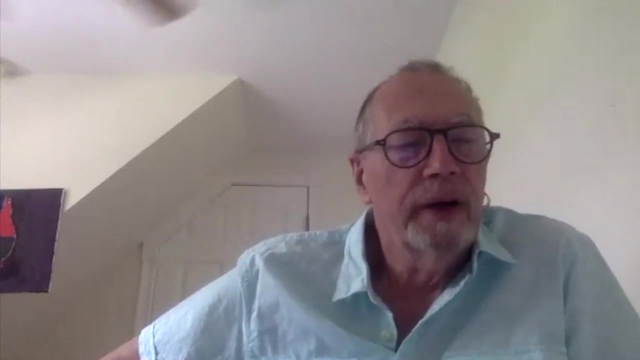 And at the end of the day the paper was still blank. So you know this was a tough issue. But around the sort of between 1905 and 1908, he played with various ideas And the one that sort of satisfies him eventually. 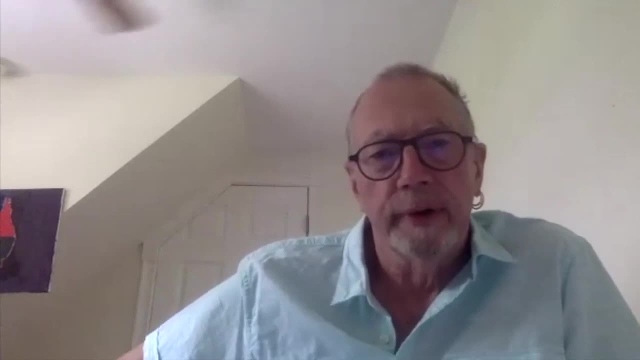 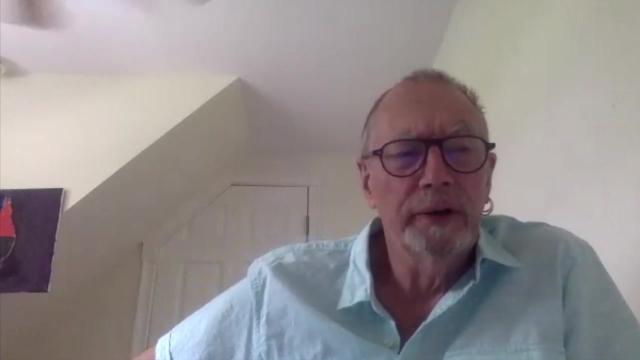 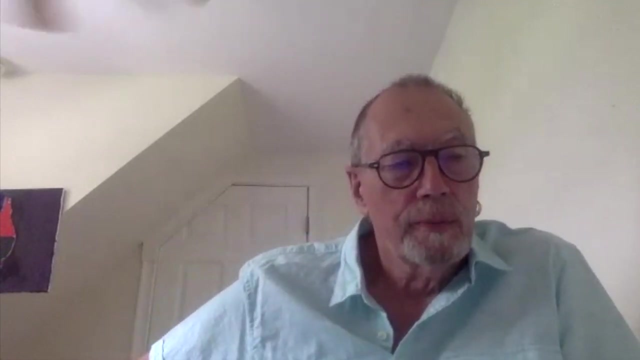 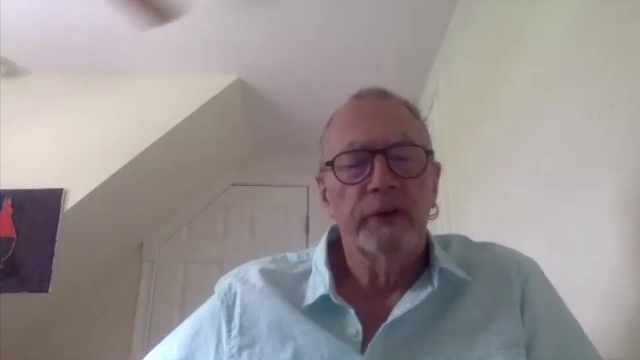 the one that appears in Principia is called type theory. Now type theory itself can be formulated in various different ways. Let's take the simple version first. The thought is that you've got to rank mathematical objects in a hierarchy. So at the ground level, 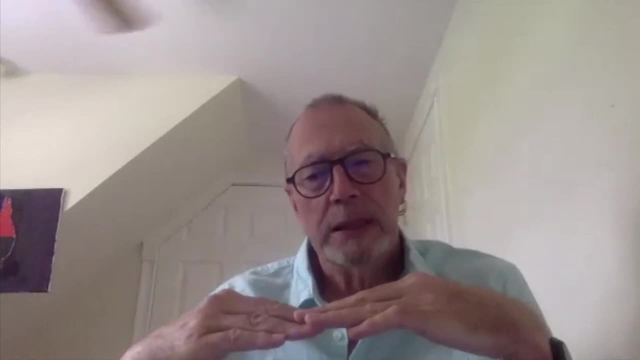 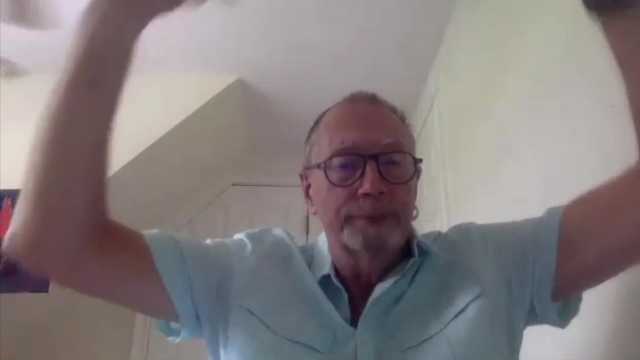 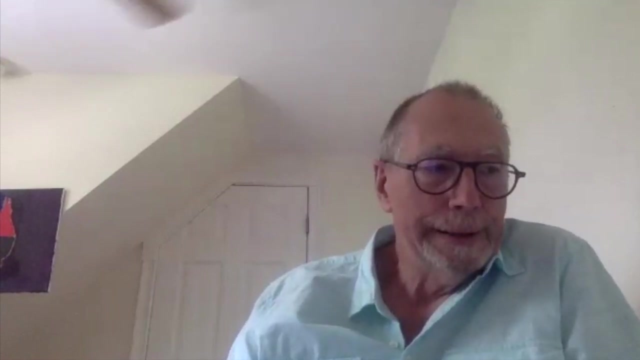 you have maybe just ordinary concrete objects. Then the next level up, you have sets of those and then sets of sets of those, and then sets and sets of those, all the way up, Whatever that means. So you take it as a given. 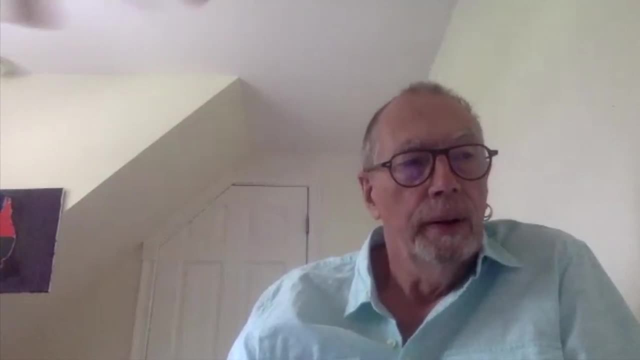 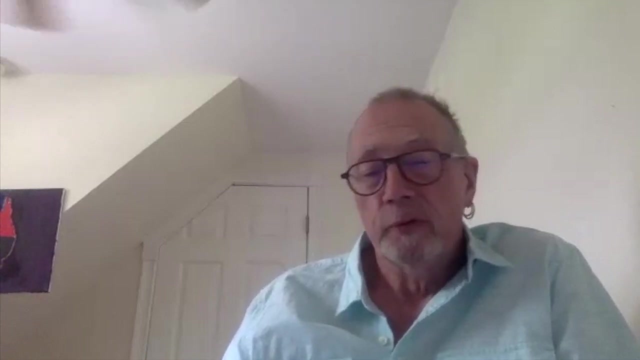 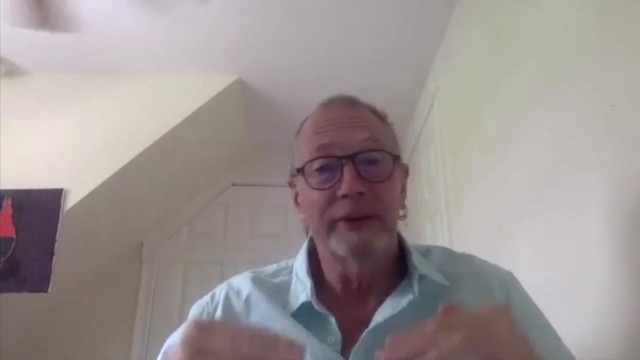 that sets have this hierarchical structure And if you dig your heels in and insist that, then you can avoid Russell's paradox, Because according to Russell, you can't quantify over all these sets. What you can do is quantify only over sets of some level. 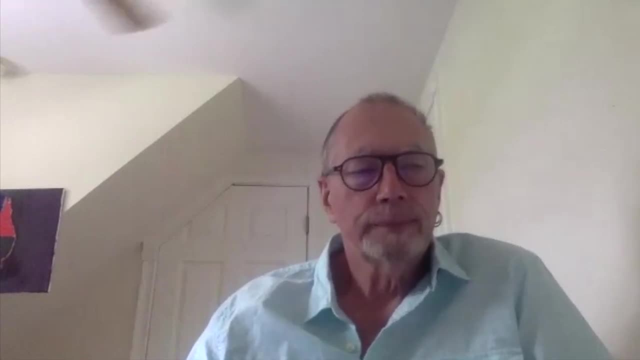 So if you want to say that a set of level n is a member of set of level n plus one, you've got two types of variables: those subscripted by n, those subscripted by n plus one. And you can say things like: 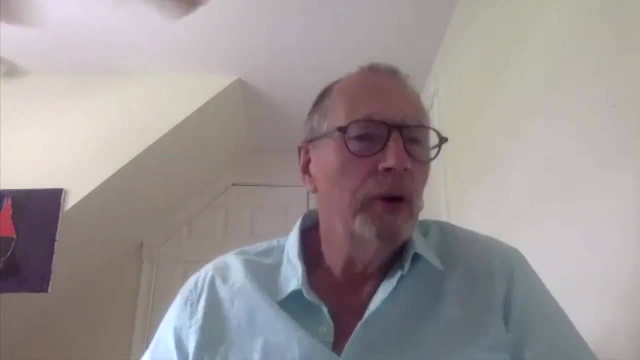 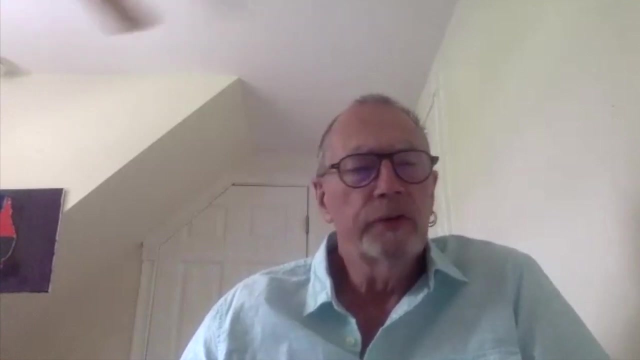 xn is a member of xn plus one Now. but if you look at Russell's paradox, you need to say that x is a member of xn plus one, But x is a member itself or not a member itself, And this is just ruled out by the syntax. 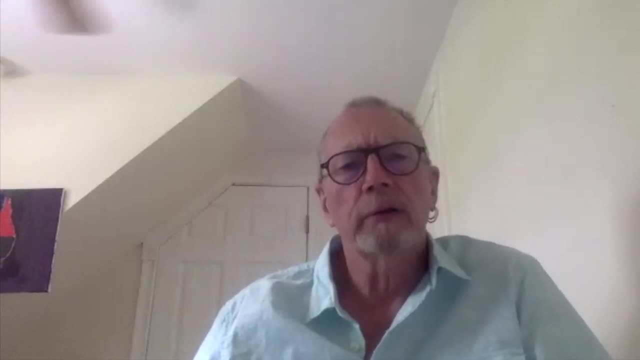 So you can't even formulate Russell's paradox. It turns out to be ungrammatical. So this was Russell's solution. It has a number of unlovely features. The first is that you've got this reduplication of levels. 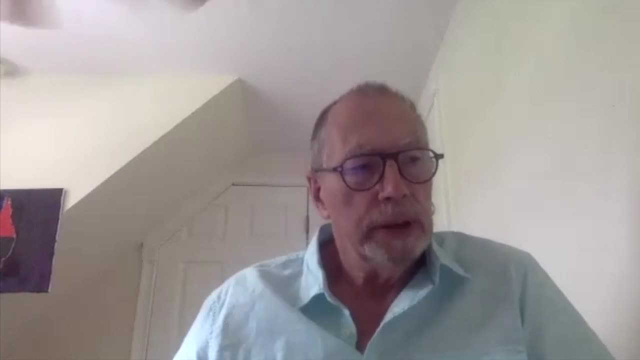 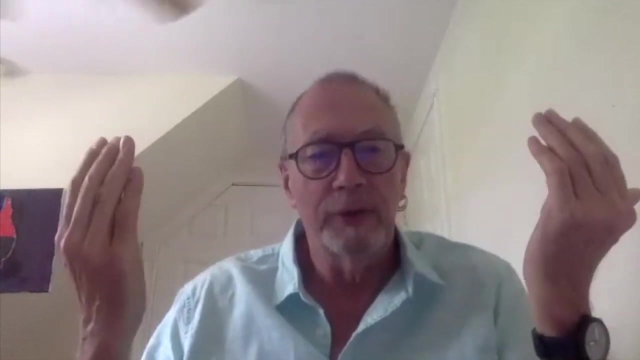 So if your aim is to construct numbers, you're going to get an infinite repetition. You're going to have numbers at level. I think the first level they appear at is level three. Then you're going to have the same like have numbers at level four and five and six. 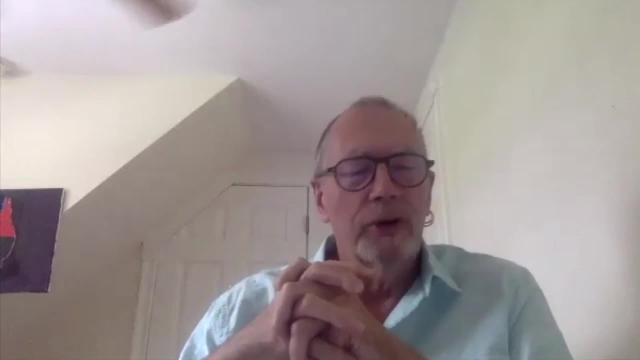 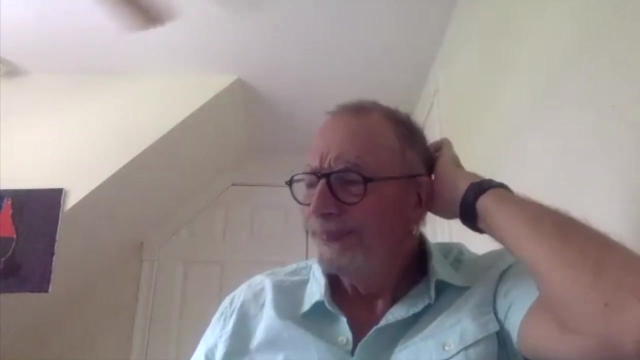 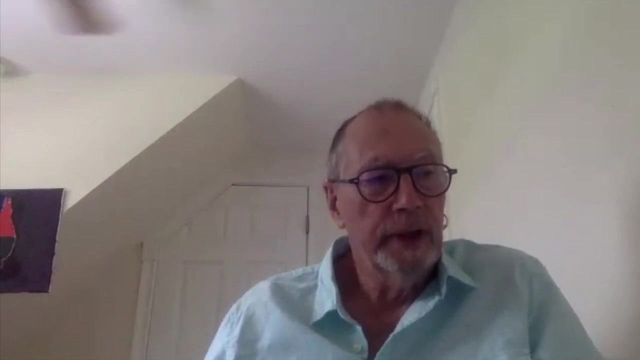 So you've got this infinite reduplication. It's not clear that's a knockdown problem, but it's certainly, as I say, unlovely. Another more worrying feature is this: A nice aspect of Frager's account was that you're actually able to prove 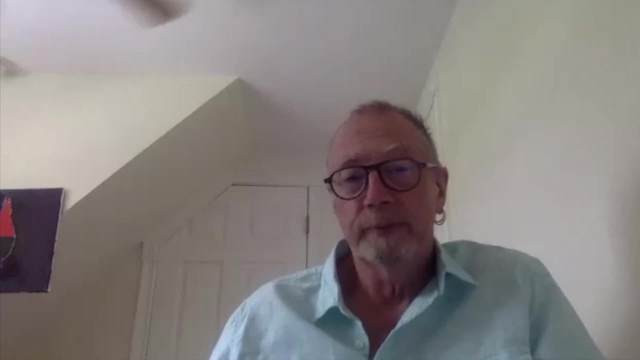 that there's an infinite number of objects. So you can do this kind of argument: Take an object, then take its singleton, and the singleton of that, and the singleton of that and so on. That's going to be an infinite number of different sets. 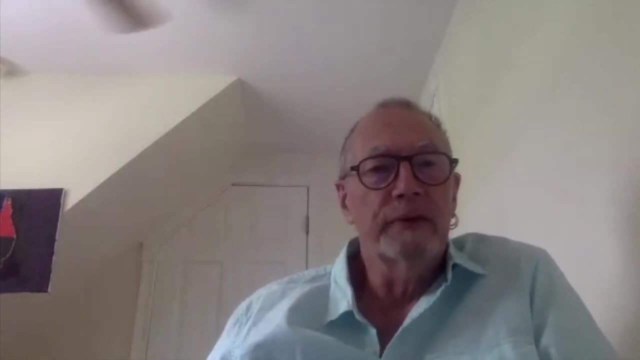 Okay, So with a bit of fiddling you can turn that into proof that there's an infinite set in Frager's theory. You cannot do this in Russell's theory. I mean, you can have an object, It's singleton, it's singleton. 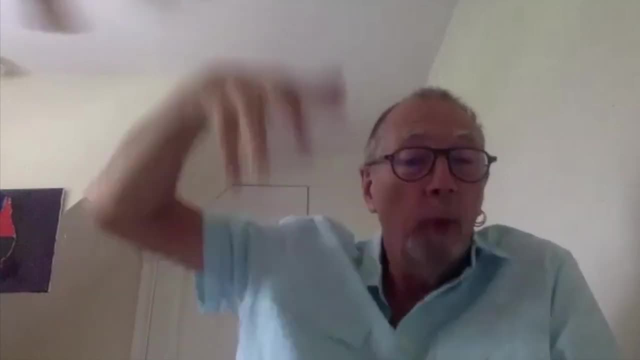 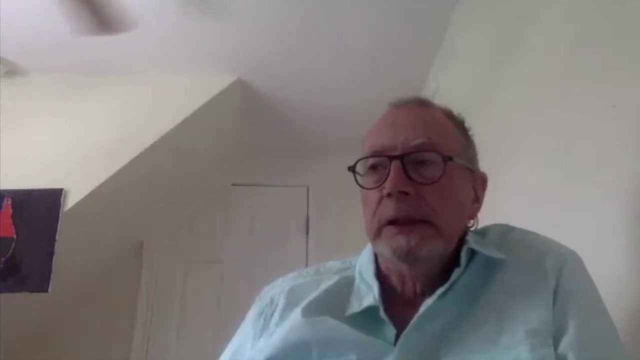 but it's singleton and so on all the way up. But this whole bunch of things isn't a set of any particular type. It goes through all the type hierarchy And so there's no way in Russell's system you can prove there's an infinite number of things. 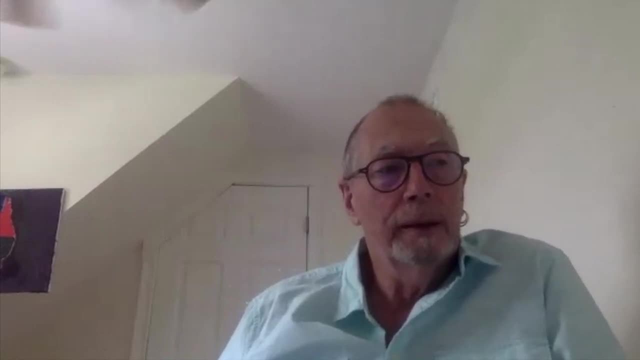 And if you can't do that, then you can't do mathematics. So Russell was forced to take as an axiom something called the axiom of affinity, which is essentially an axiom that there's an infinite number of objects at the ground level. 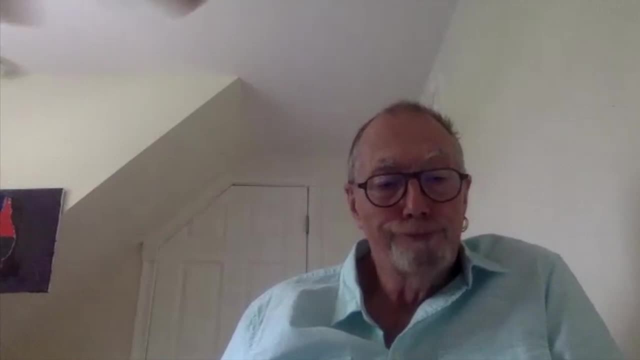 And if you're thinking of those as physical objects, then it's not clear. that's true, But even worse, it doesn't look like it would be a fact of logic. I mean, there's a logically possible world in which there's only one object. 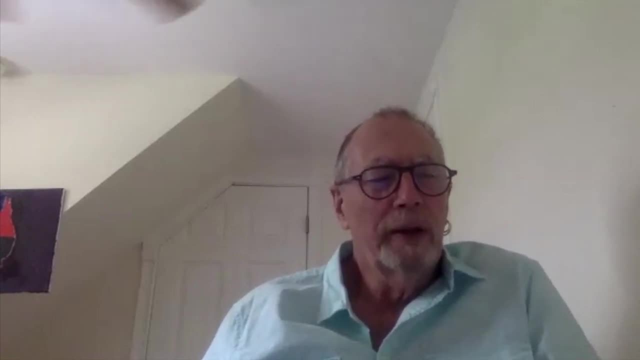 So this was one of the problems that he had to deal with. He had to deal with axioms. for him, He seemed to have to appeal to axioms which were not logical. There's a third problem, which is more technical. This wasn't the only axiom of a non-logical kind. 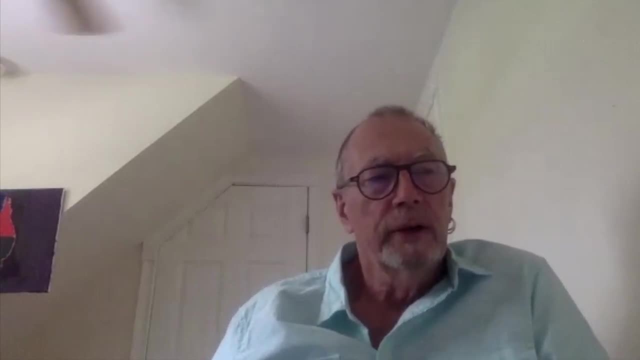 that Russell seemed to need. But the reason he needed it was because the system of type theory that he was dealing with, as I've suggested, he wanted to solve not just the set theoretic paradoxes but also the semantic paradoxes, like the liar paradox. 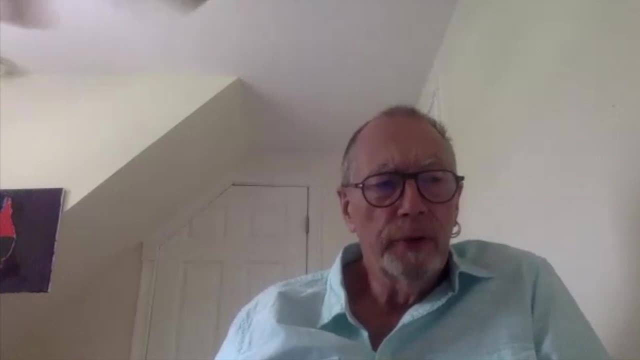 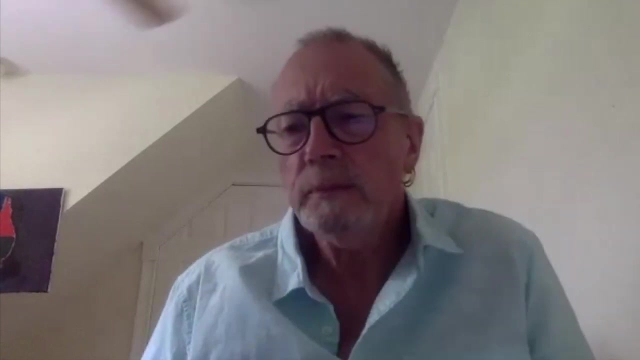 Now, if you want to do that, this set theoretic structure on its own is not good enough. What you've got to do is take into account not only the level of sets, but the level of how things are defined, the specification of a set. 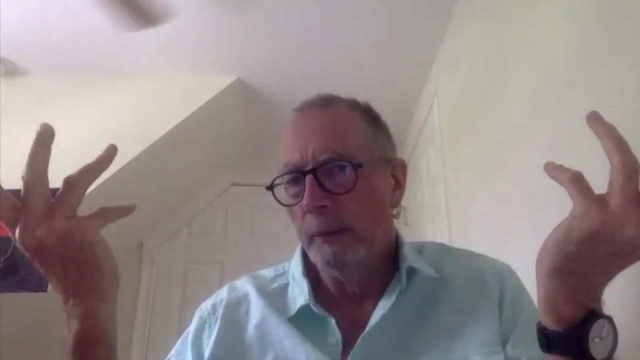 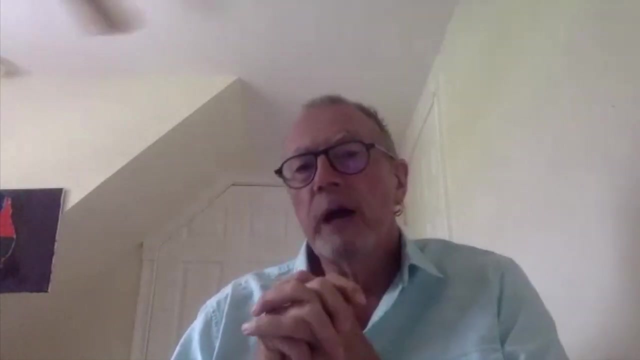 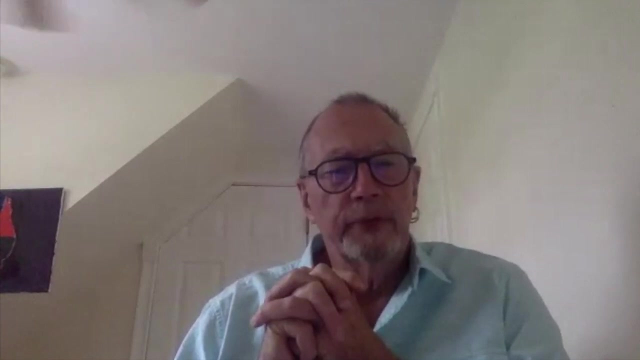 And you've got to form those into a hierarchy as well, And this makes the structure much more complex. This is sometimes called the ramified theory of types, And if you try to work in a ramified theory of types, it messes up a number of mathematical proofs. Because when you give the definitions of sets, they turn out not to have the right level. So you need an axiom to say, well, okay, this thing you can't show it has the right level, but we take it as an axiom. 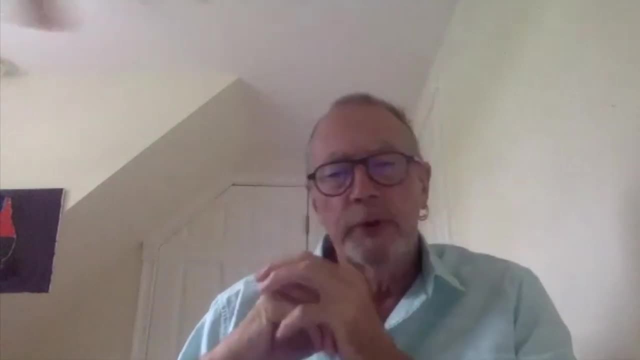 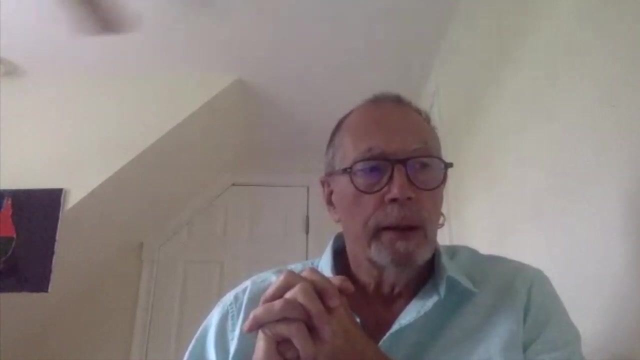 there is something of the right level. This is called the axiom of reducibility- And again, Russell was not happy with it, So this was another problem that he faced. Now, there's a bit of interesting history here, because when early logicians and philosophers 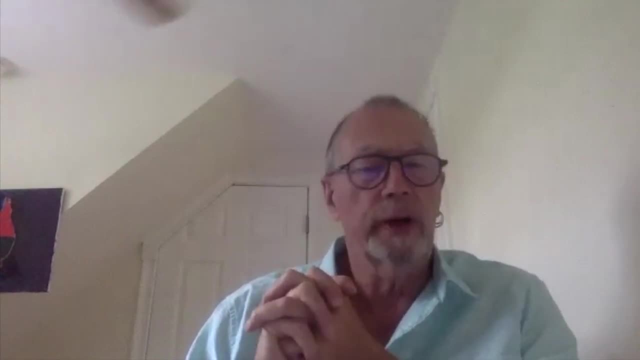 took up Russell's work. one of them was Frank Ramsey, a Cambridge philosopher, mathematician, who died very young, the age of 28,. I think He would have been one of the great philosophers, logicians of the 20th century had he lived. 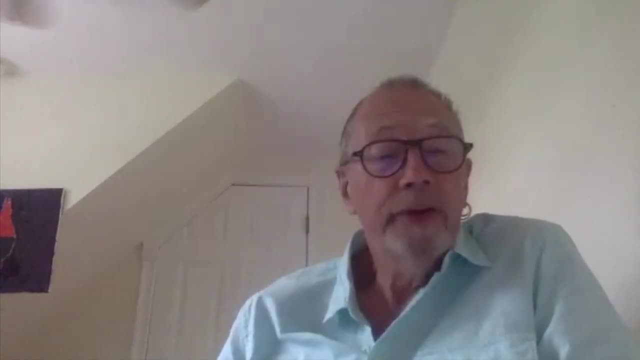 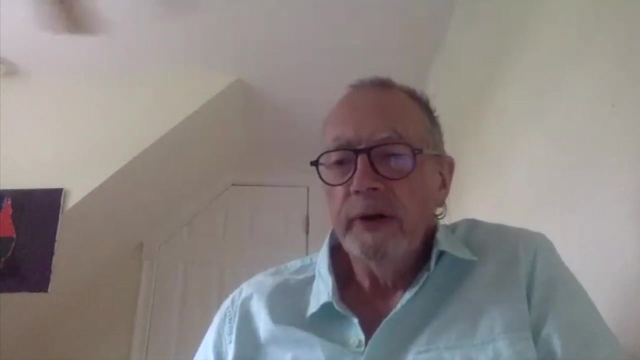 But he was one of the very few people that Wittgenstein would actually condescend to speak to. Anyway, what Ramsey did was say: look, Bertie, you don't need the ramified theory. The simplified theory is good enough for your purposes. 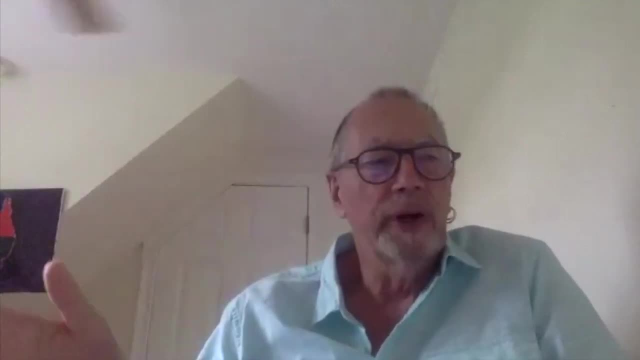 So just get rid of the ramification. We go back to the simple type that you don't need an axiom of reducibility And that's great. So in a sense, that solved the problem, Although to do this, Ramsey had to admit that. 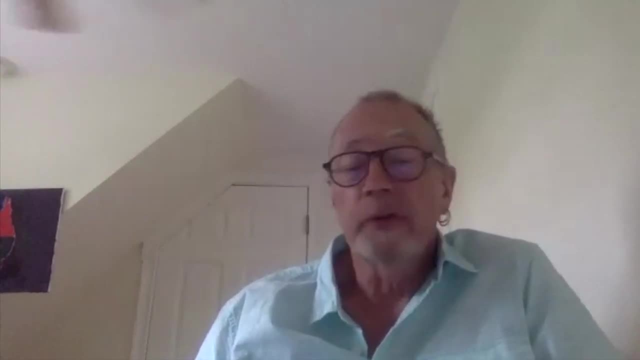 this structure would not deal with the paradox of self-reference, such as the liar, And so Ramsey had to divide the paradoxes of self-reference into kind of the set theoretic and the semantic, And so the cost of sticking just with the simplified theory was you had to do something else.